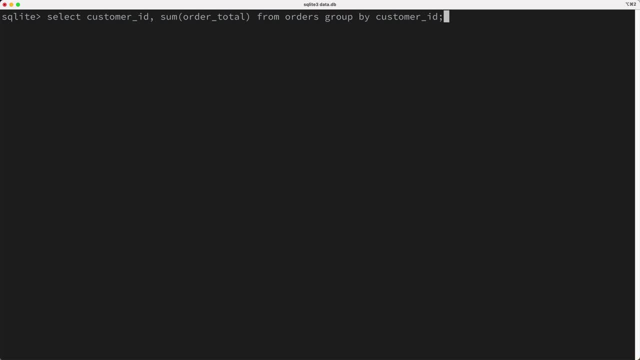 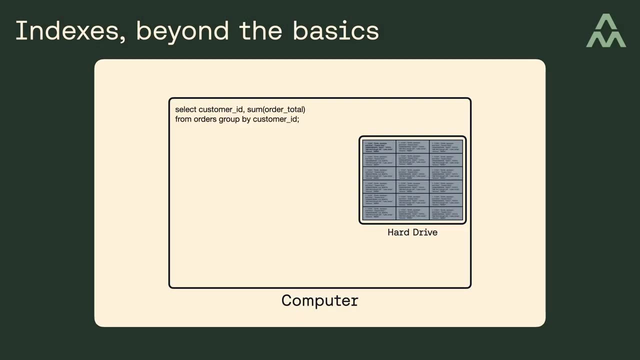 So how does the database execute this query? Well, the database is going to have to scan every single row in the table. So what does a table scan look like under the hood? Well, SQLite will figure out which database pages contain rows from the orders table. 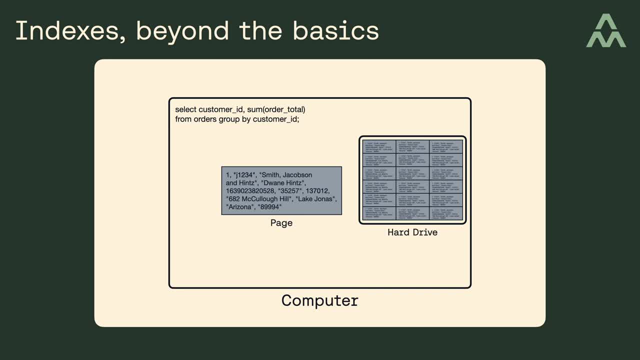 and those pages will get pulled off disk and the customer ID and the order total will get pulled out of the page and used to satisfy the query. And this process of fetching a page and pulling the needed values out of the page repeats over and over until all the order data is retrieved. 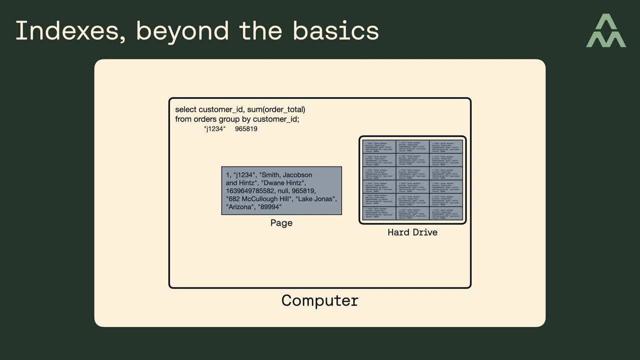 Now, did you notice any inefficiencies in what I just described? The inefficiency I'm referring to is subtle, so I'll give you a hint: It has to do with input-output, or I don't know input-output. So do you see what I'm referring to? Well, the problem with this query is that 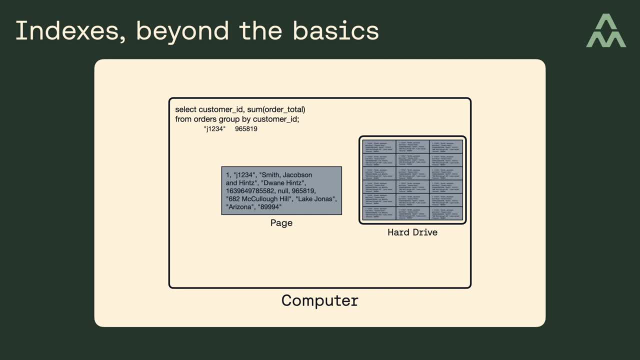 we have to pull the entire page from disk and of course pages are row-oriented in SQLite, which means database pages contain all the columns in the row or rows that are stored in the page. So to execute this query we end up having to perform I-O to fetch a lot of data that we 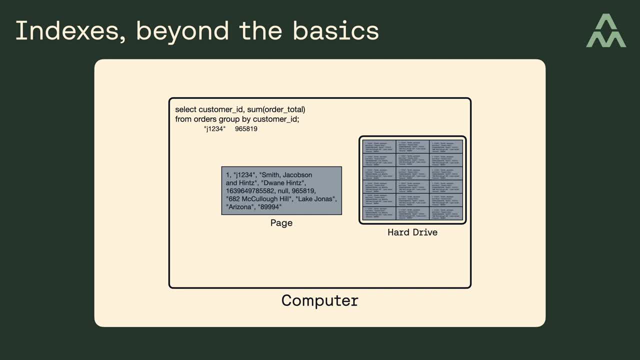 aren't really interested in. So can we improve this query somehow? Well, yeah, we can, and the solution isn't obvious. But before we try and improve the query, let's measure how long it takes to execute this query. So let's start with the query. So let's start with the query. 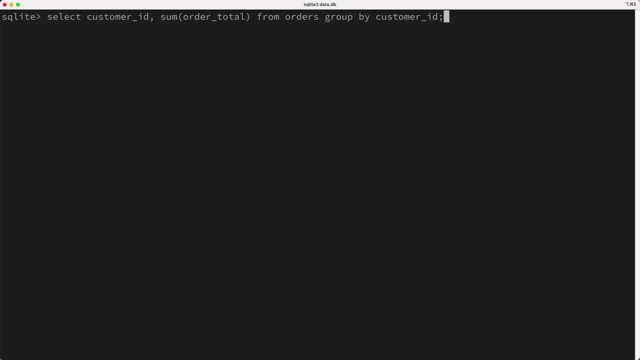 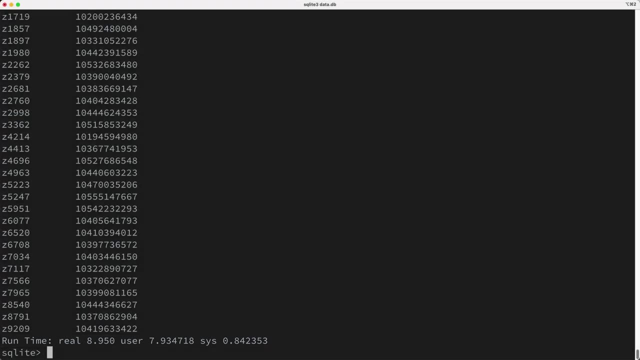 So let's try and execute this query without any optimizations applied. So I'll run this query, then I'll fast forward the video so we don't have to wait And, as you can see, it took about eight seconds to complete this query. Okay, so what can we do to improve this? 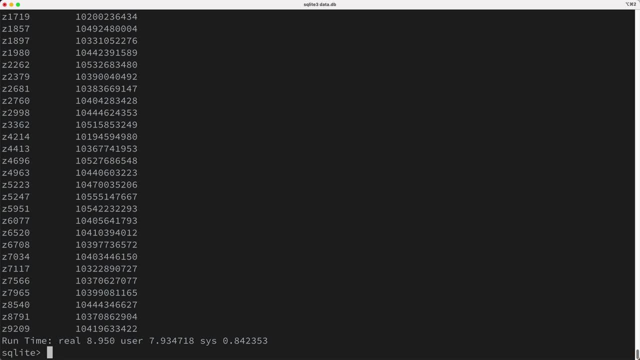 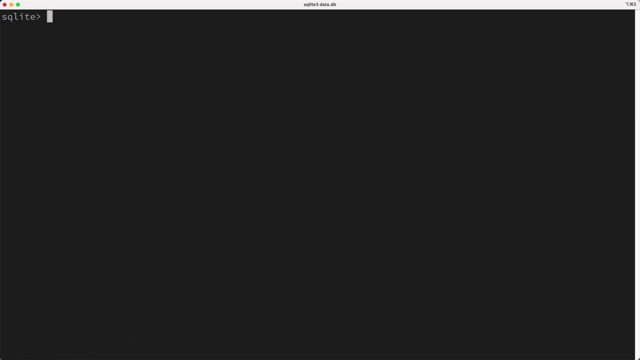 query. Well, the thing you do to improve most queries is to add one or more indexes. So we could add an index here, but would it help? Well, let's see. So I'll add an index on the customer ID. So to do this, I'll create an index named orders, customer ID- IDX on the order tables- customer ID. 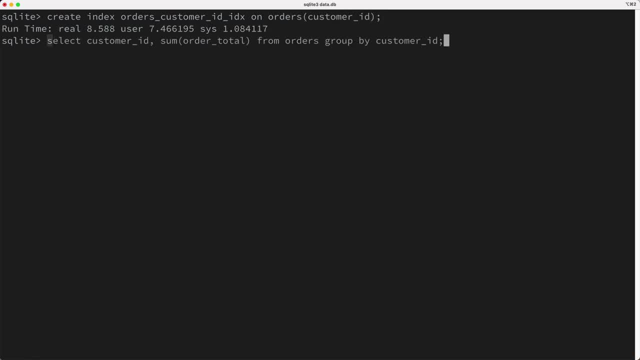 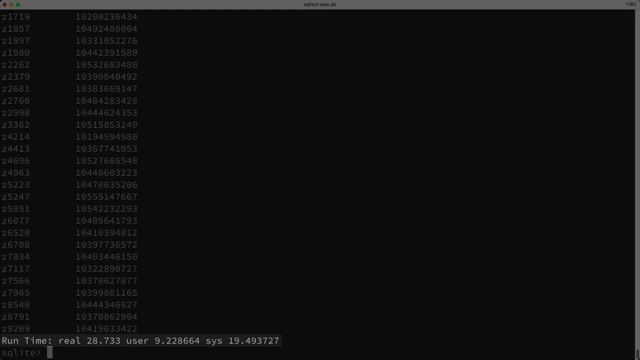 column. Ok, now we'll run the query again and I'll speed up the video. and hmm, ok, well, the query took just shy of 30 seconds. so yeah, the index we added didn't help. in fact, it seemed to make it worse. 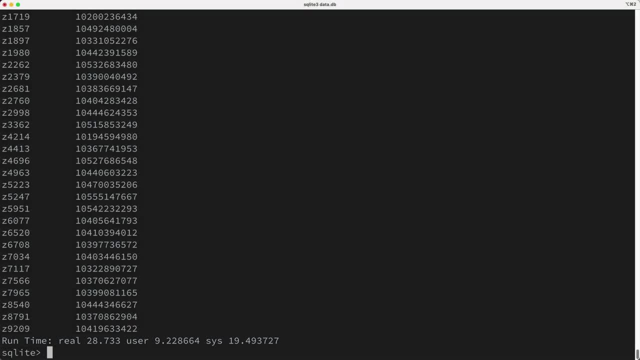 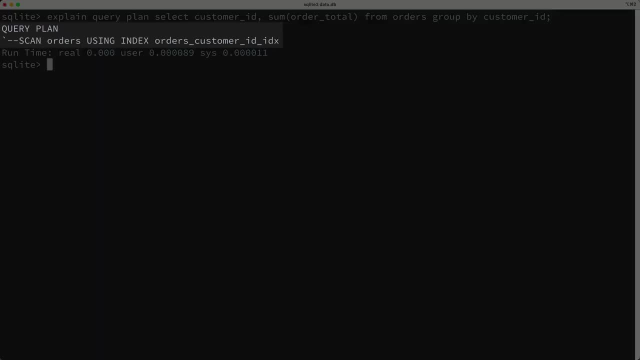 So what's going on here? Well, it seems like the query planner picked an inefficient solution and if we run the last query again- but we pre-pinned explain query plan- you see that a scan of the orders table is occurring and it's also referencing our new index. 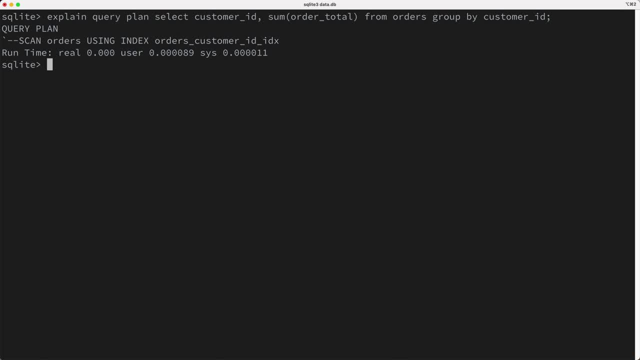 So, basically, our query is reading every page from the orders table and it's reading our new index for some reason, and it's probably jumping back and forth between the index and the table data. Ok, so should we get rid of the last index? 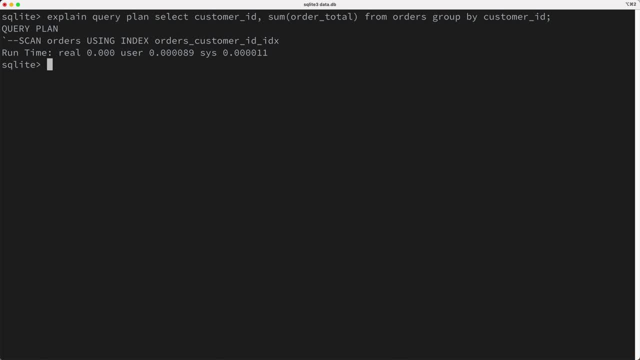 Well, probably not, because it seems very likely that other queries will need to search by the customer ID, as that's pretty common. so are we stuck or is there something else we can do? What if we created another index that includes both the customer ID and the order? total columns. 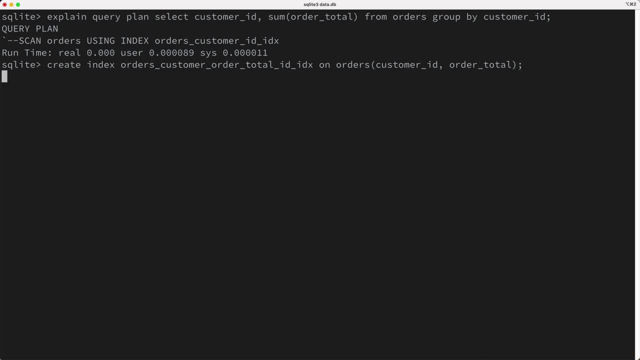 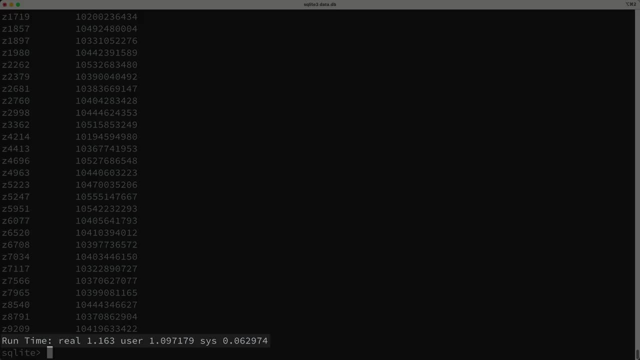 Would that help our query? Let's try and see. So I'll create our new index on both columns, as you see here. Now I'll go ahead and run our query again and check that out. Our query finished in about one second, which is about 30 times faster than the last time. 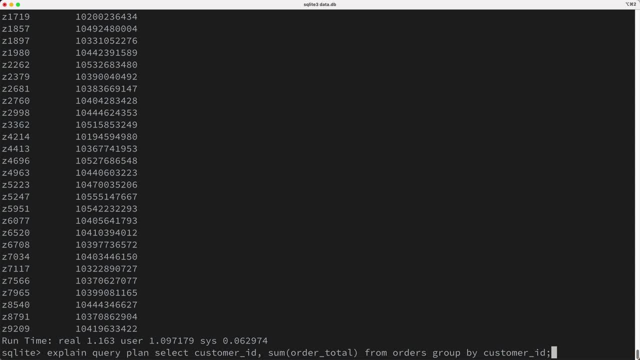 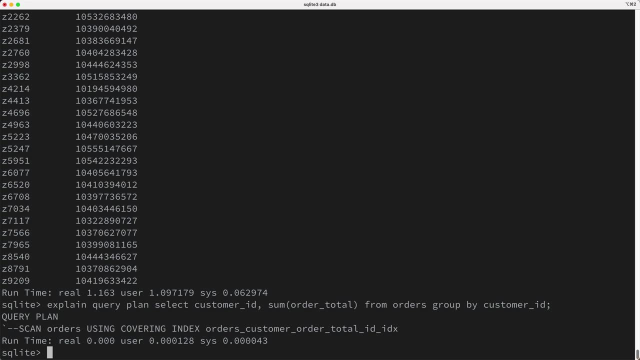 we ran this, Ok, I bet this result is surprising to some of you. So how is it that this index helps our query? Well, it helps, because this index can now be used as the source of data for our query. In other words, our index contains all the data needed to calculate the result, and so 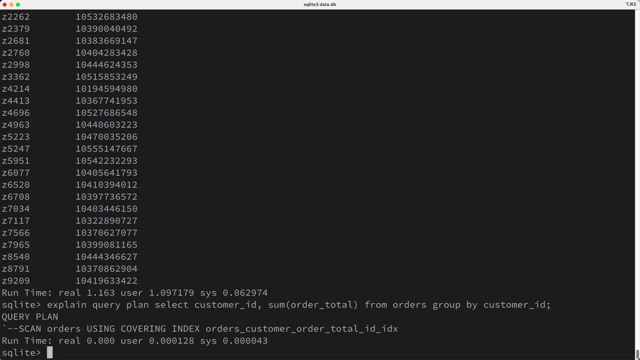 we don't need to scan the order table. We can just scan the index to calculate the result. So why is it more efficient to scan the index instead of the table? Because when we're pulling the pages for the index, we're getting just the data we need. 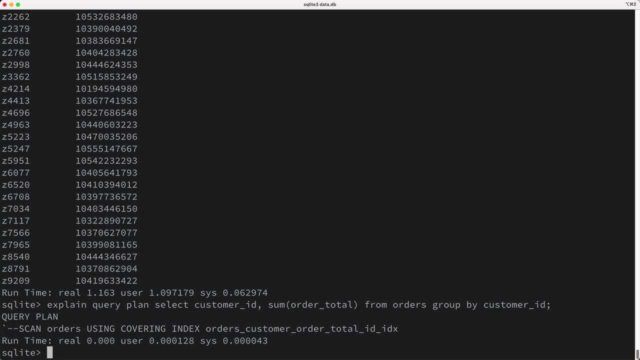 We're not having to pull all the unnecessary data, as happens when you're doing a table scan, like we saw earlier, So there's a lot less IO that needs to happen to calculate the result. There's a name for this kind of an index? 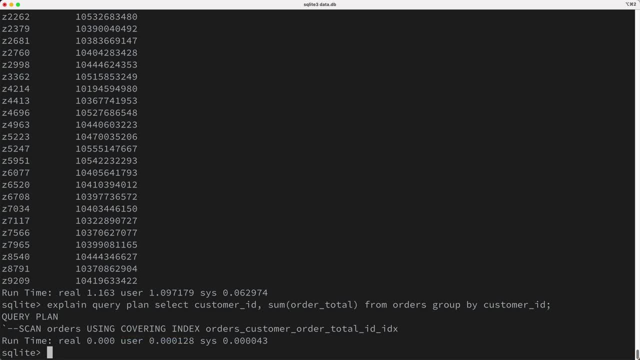 It's called a covering index. So is adding this index a good idea? Well, that's a judgement call, And here are the things you need to consider. First of all, is this a query that is frequently used? If you do use this query regularly, then adding this index might be the right choice. but 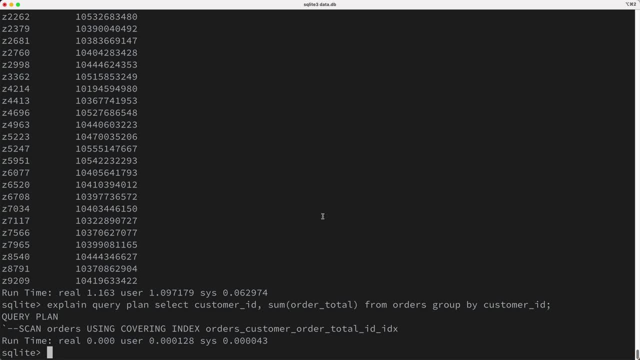 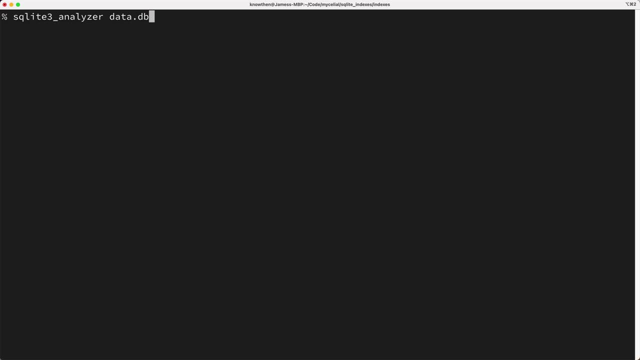 there are tradeoffs that you need to keep in mind. For example, halving this index takes disk space, and we can see how much disk space is used by using the SQLite 3 analyzer, which is installed by default with the SQLite command line interface. 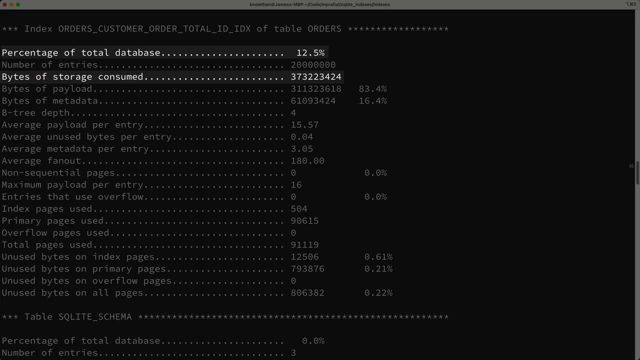 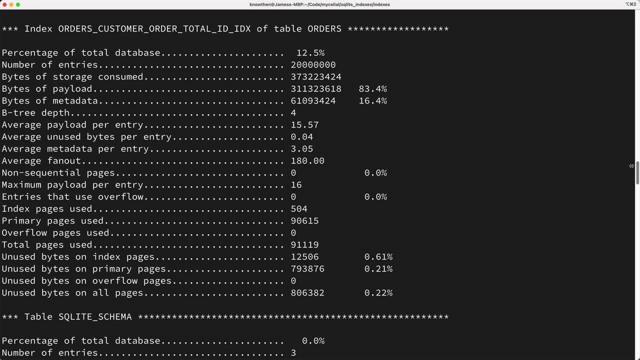 And, as you can see here, this new index consumes about 12.5% of the total disk space, So that's a good thing. Now, if we've got plenty of disk space, then halving this index could be totally fine. but disk space isn't the only concern. 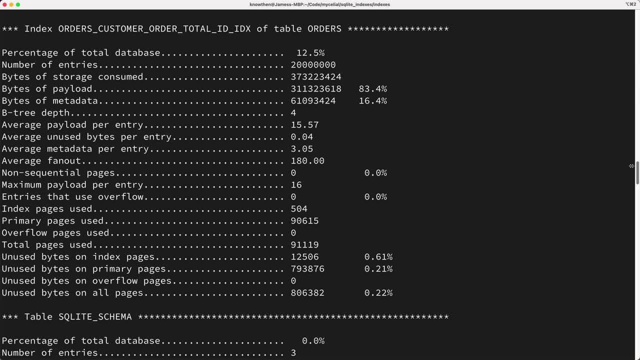 The other relevant concern is that the more indexes we have, the worse the performance of mutations. In other words, inserts, updates and deletes can take longer to complete because the indexes need to be updated on every mutation. So should we keep this index? 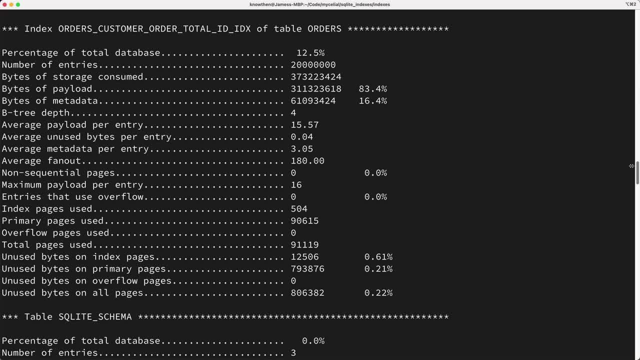 Well, again, it's a judgement call, but the more important thing for you to know is that covering indexes can be updated on every mutation, So let's go ahead and do that. First, let's take a look at an example of a query that can result in greatly improved 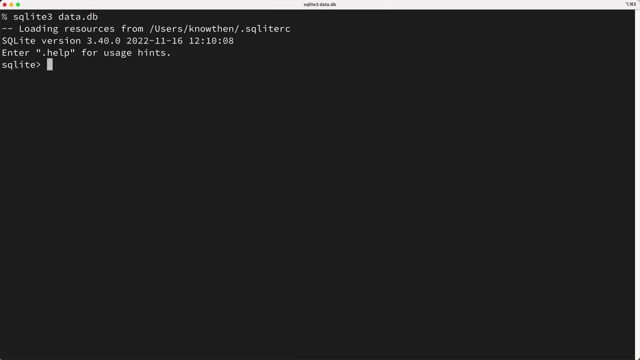 queries and it's a tool you should have in your tool belt. You know, a common query that happens against this orders table is to query for an order by its purchase order ID. So, for example, here's a fairly common query for an order by the purchase order number. 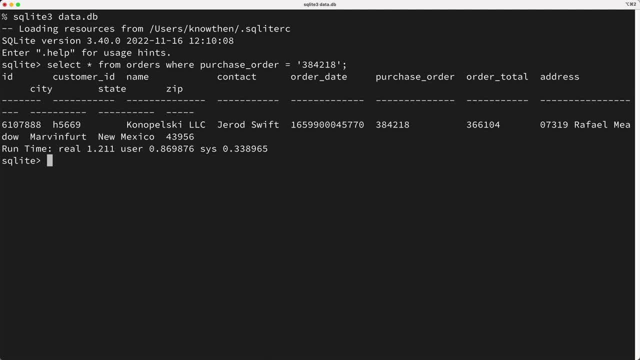 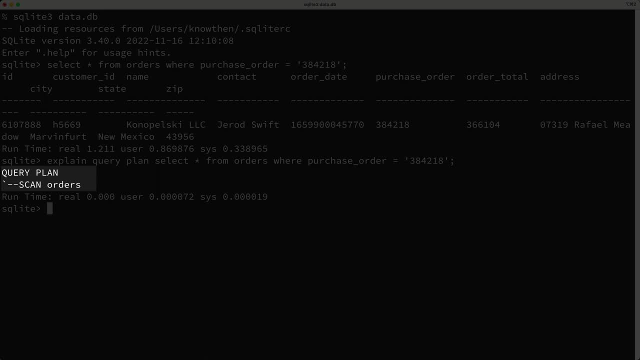 Now, as you can see, this query is pretty slow and if we prefix the query with explain query plan, we see it's slow because it's doing a full table scan of the orders table. In other words, it has to look at all 20 million rows to determine the result. 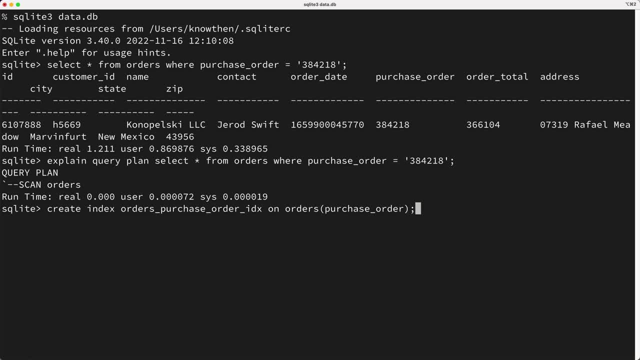 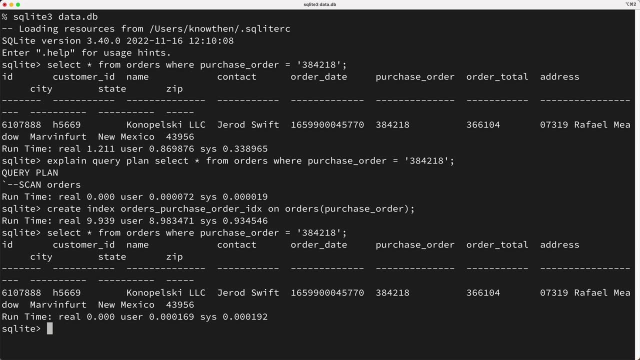 So let's go ahead and add an index on the order table's purchase order column And if we run the query again, it completes almost instantly, which is great. but I want to point out something about the purchase order column. If you look at a few records, you'll notice that the purchase order column is null for. 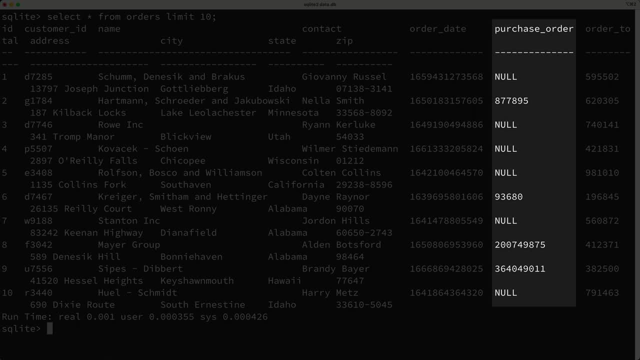 a lot of rows. So do you see any potential problems with the purchase order index we created, considering the fact that there seems to be quite a few null values in this column? Well, the problem is that the null values are included in the index, but users don't. 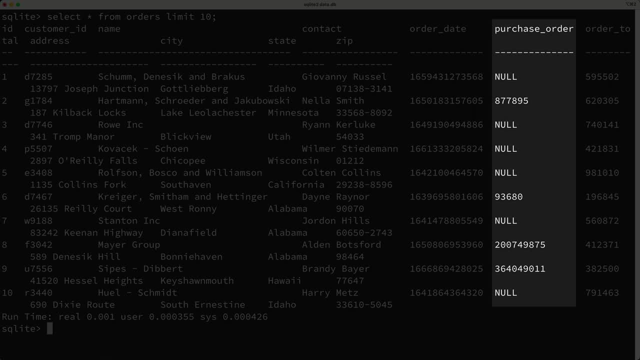 routinely search for null values. When users search for null purchase order values, usually they search for a specific purchase order number. So what does this mean? Well, it means that our index is using space to store null values, which is wasteful because 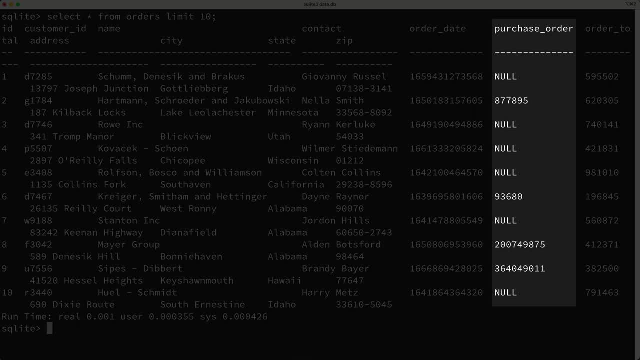 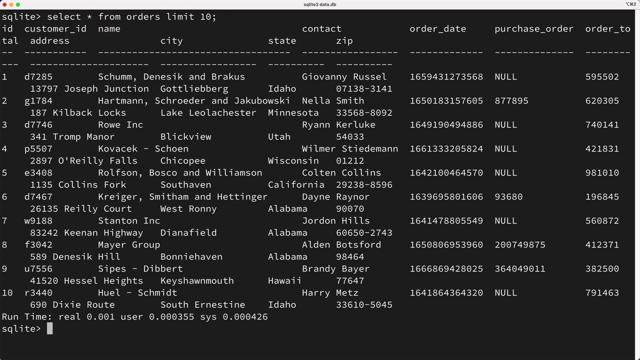 users don't search for null purchase orders, So is there any way to save the wasted disk space that's consumed by null values? Yep, there is. We can change our index to be what's called a partial index. But before we fix our index, let's look at the current size of the index, which includes: 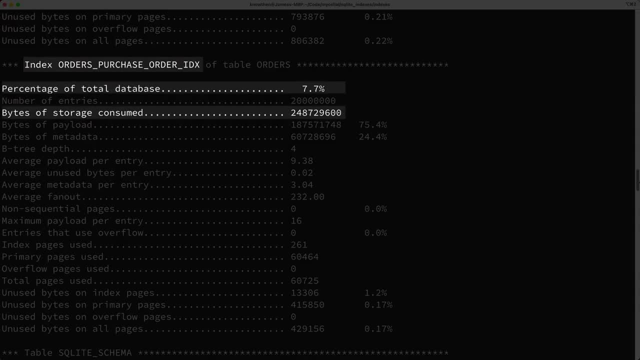 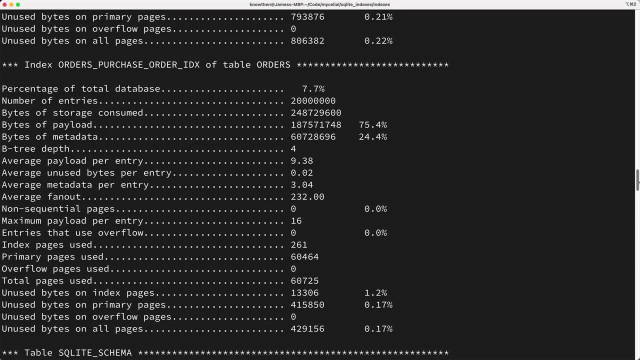 the null values And, as you can see here, the index consumes about 7.5.. That's about 0.7% of the disk space, which is about 249 megabytes in size. Okay, so how do we fix this index? 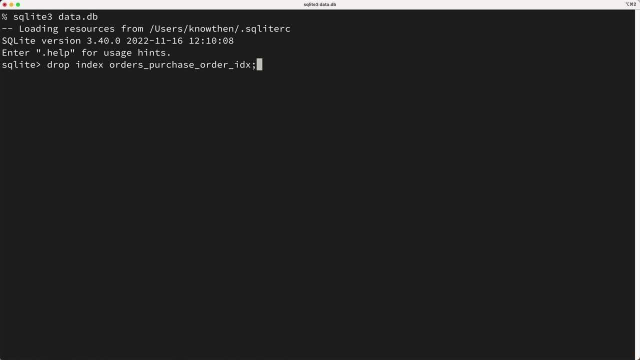 Let me show you. First I'll drop the purchase order index, then I'll create a new index, just like we did a moment ago, but I'll add a where clause which specifies that the index should be created only when the purchase order is not null. 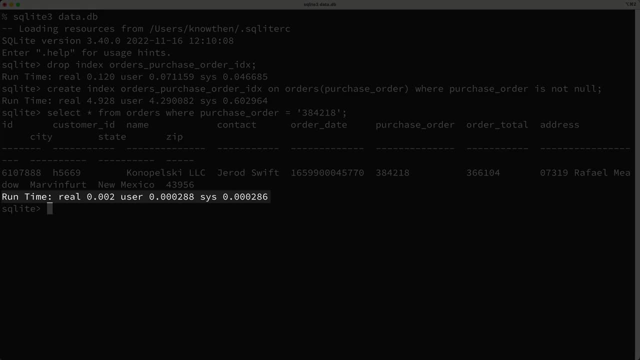 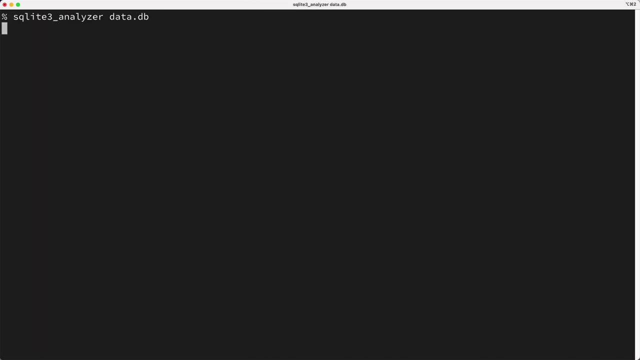 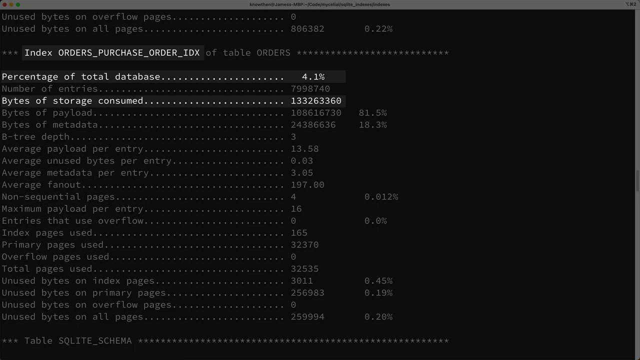 Now I'll run our purchase order query again and, as you can see, it executes just as fast as before. So let's take a look at how much disk space our new purchase order index takes And, as you can see here, it's down to about 4.1%, or 133 megabytes in size. 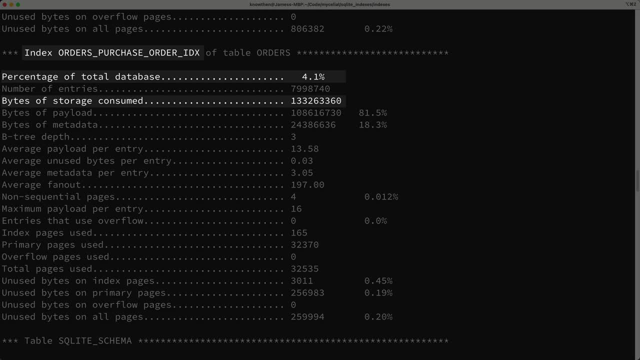 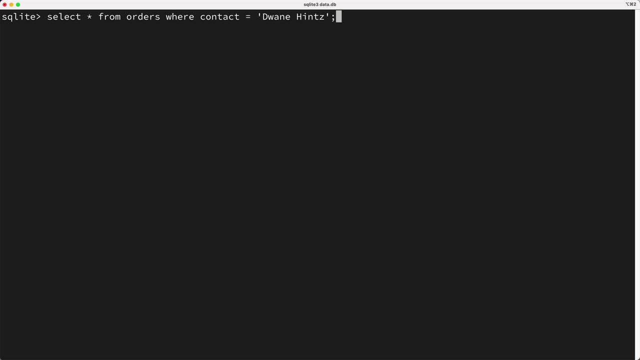 So we were able to nearly halve the amount of space used by our purchase order index without any compromise in performance. Nice, Okay, there's one more type of index I want to look at. So sometimes users query the orders table by the contact name, like this: 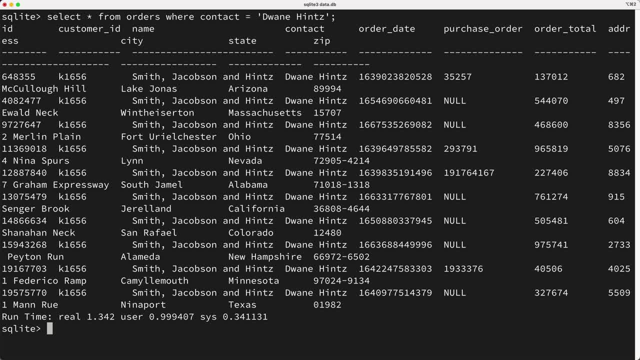 But this query is case sensitive and often the users don't get a result from this query because of this case sensitivity. For example, if I query for this contact in lowercase, I don't get a result because, again, it's case sensitive. 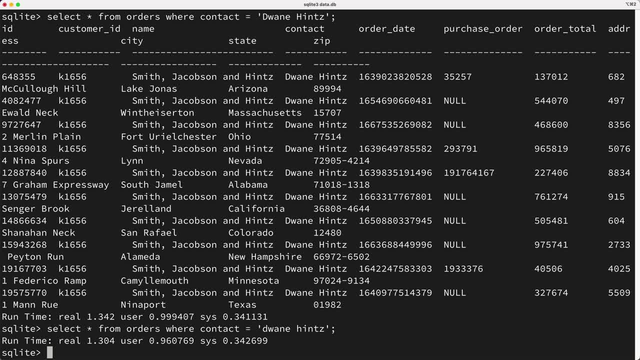 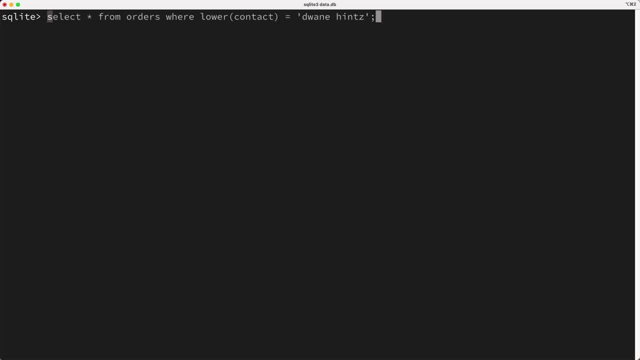 I'd like to make this query a bit more friendly and forgiving. In other words, I'd like this query to work in a non-case, sensitive way. So do you have any thoughts on how we can accomplish this? Well, what if we did this? 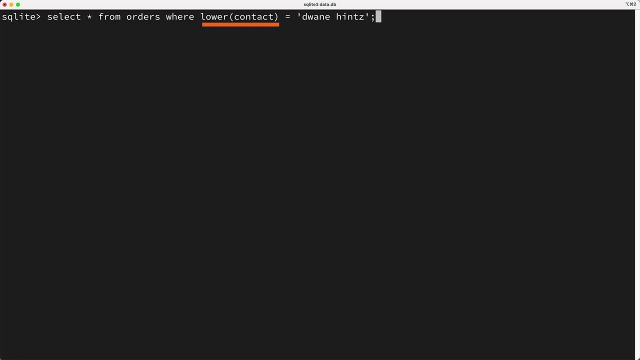 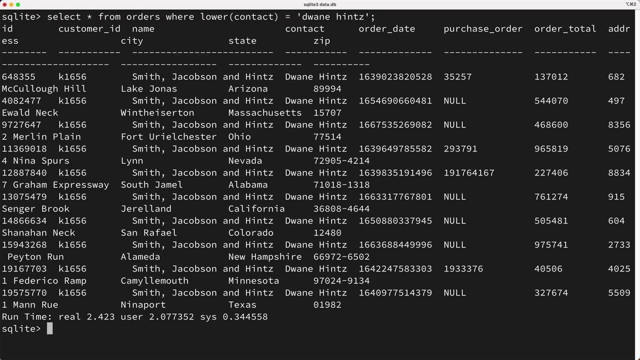 We query for the order where the lowercase version of the contact column matches our lowercase name. So this works, but it's not a very efficient query. Do you see why? Well, the problem is Because where we call the lower function has to be called on the contact column of. 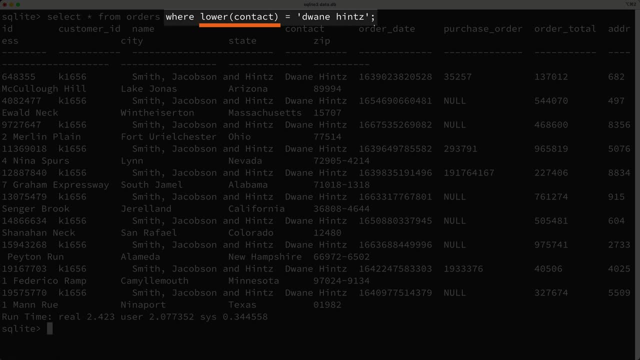 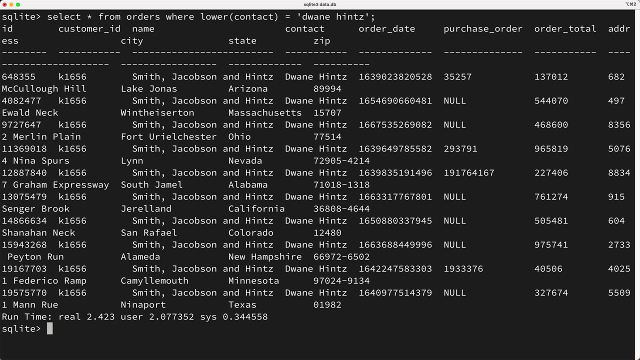 every single row in our table to properly evaluate this entire expression so effectively. this query has to perform an expensive table scan to get a result. So how do we fix this? Well, we have to add an index on the contacts column right. 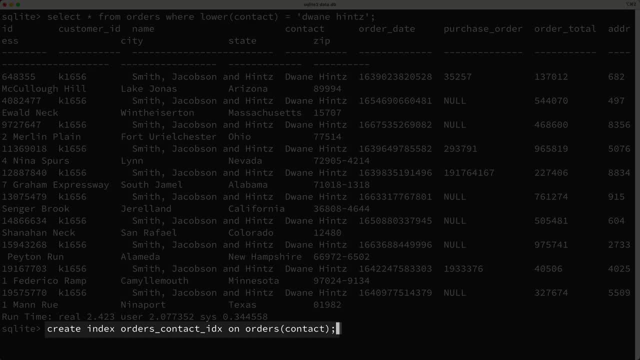 So do you think this create index statement will work for us? Hmm, well, let's try it and see. So I'll add the index and I'll run our query again and, as you can see, it's still a really slow query. 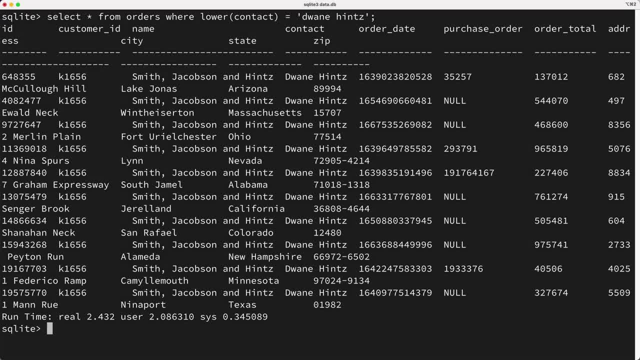 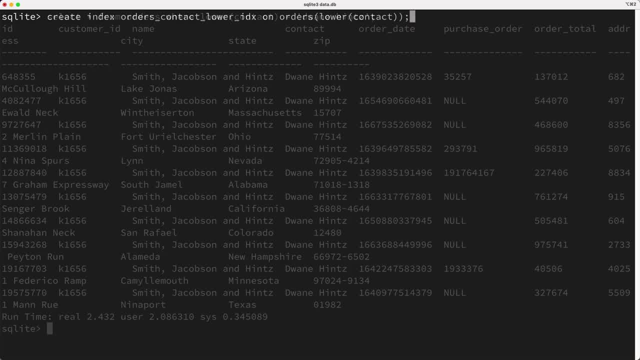 So why didn't this query work? Why didn't this index work for us? Well, because it's indexing in a case-sensitive way. but there's a trick we can perform where, instead of indexing on the contacts column, instead we index on the lowercase version.